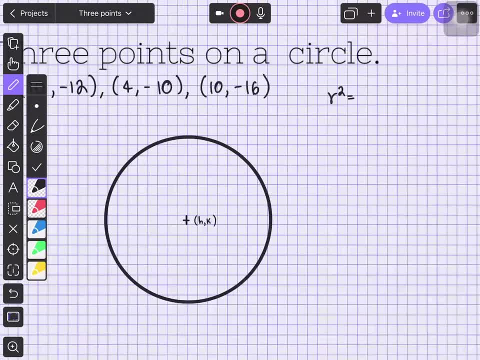 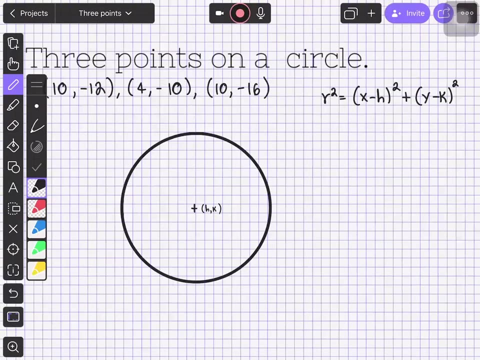 We know that the equation of the circle is defined as: r squared equals x minus h squared, Plus y minus k squared. all right, But we don't have the radius and we don't have the center, all right. So the idea is this: 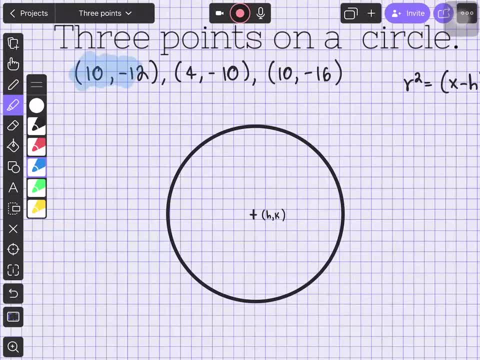 Let's identify first these points. Let's call this one here the blue point, Let's call this one here the red point, And let's call this one here the green point. Now, the precise location doesn't matter. What matters is that let's imagine the blue point is in here, the red point. I'm sorry about that. the red point is in here and the green point is in here, okay. 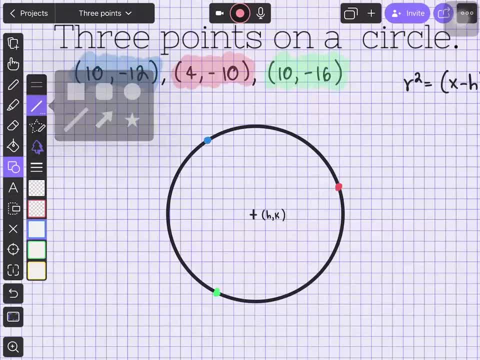 What matters is the following: Okay, This one right here. this distance from that point to the center is the radius. The distance from From this red point to the center is the radius as well, And the distance from this point, the green point, to the center is also the radius. all right, 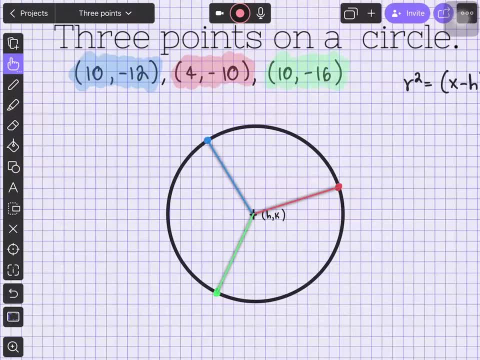 There we go, And if all of, if those distances, all of them are the radius, then this one, the blue one, the red one and the green one, they are identical And that's the principle we're going to use to solve this problem. 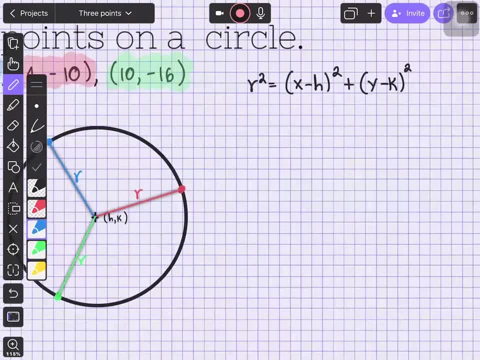 So in other words, the square radius, the blue square radius, is identical to the red square radius. So we use the formula x minus h squared, plus Y minus k squared equals x minus h squared plus y minus k squared. 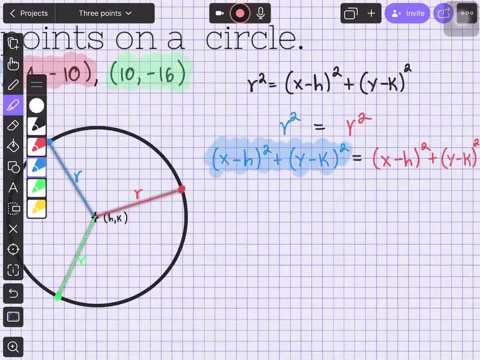 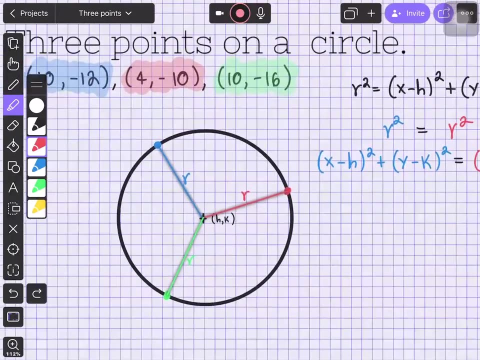 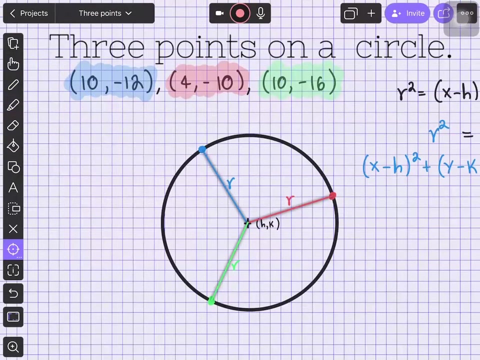 If you see, this is the blue radius, in the same way that this is the red radius, And we do have some information, And we do have some information about those equations. In this case are the coordinates for x and y of the blue point and x and y for the red point. 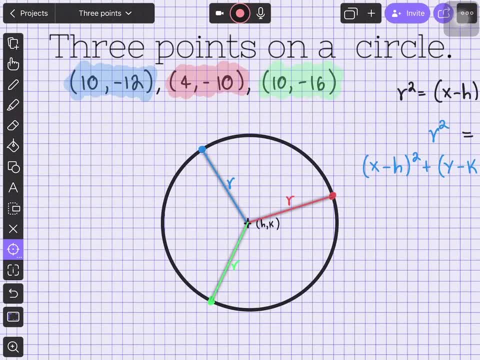 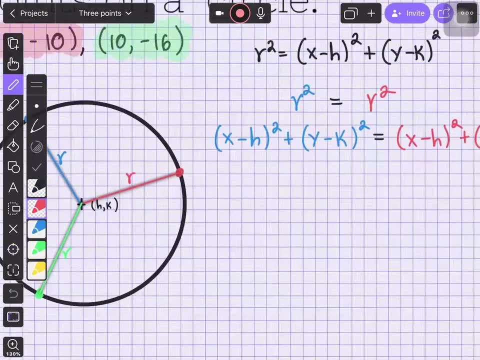 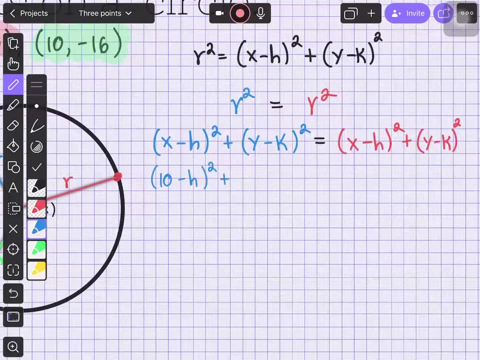 So, based on that idea, we're going to substitute those values to the equation. So 10 and negative 12 in here Once again: 10. 10. 10. Minus h squared plus negative 12, minus k squared equals. 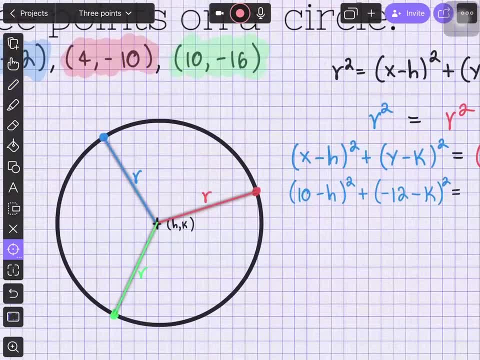 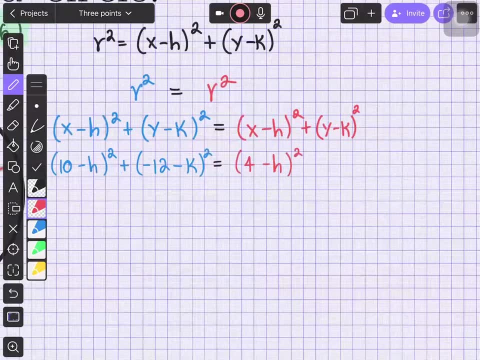 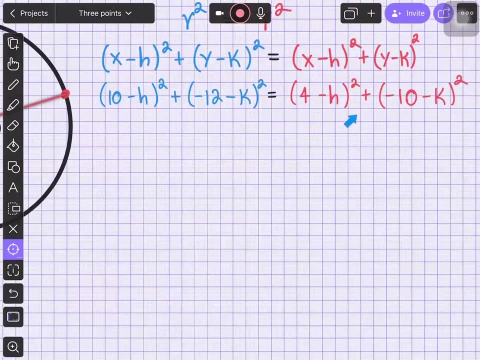 And now we do the same. All right, 4 and negative 10.. 10.. 4 minus h squared, plus negative 10, minus k squared. So now, if you see, We have 4 binoms, All right, 1,, 2,, 3 and 4.. 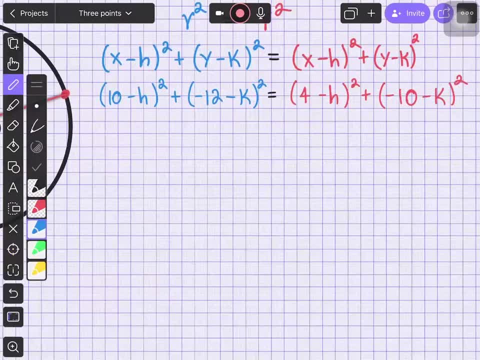 And we're going to develop them. So let's begin. We have 100, minus 20h, plus h squared plus 12 squared 144.. We both times 2. And we're going to shoot that off. That's not showing 1,, 2,, 3, and 4, and then it's not showing 1,, 2,, 3, and 4.. That's not showing 1,, 2,, 3, and 4,, which is positive. 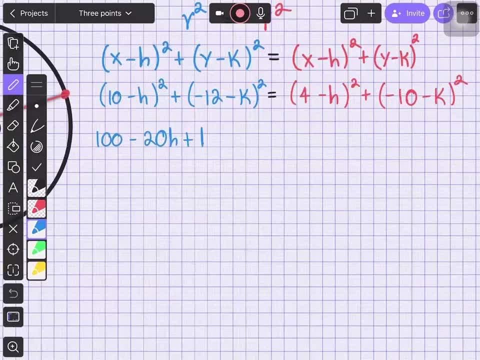 We're going to look at the real reason for that. It's because remember. It's because remember, If you count them manually, how many times can you get plus h squared, plus 12 squared 144? equal times 2, 24k plus h squared- all right, this over here is the first binom. 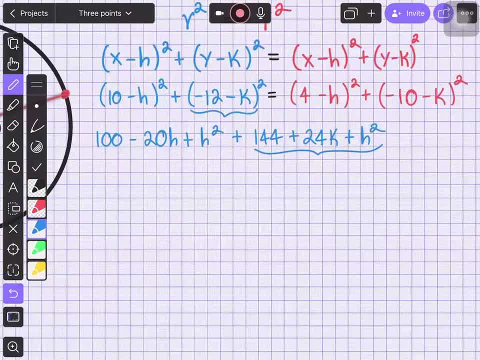 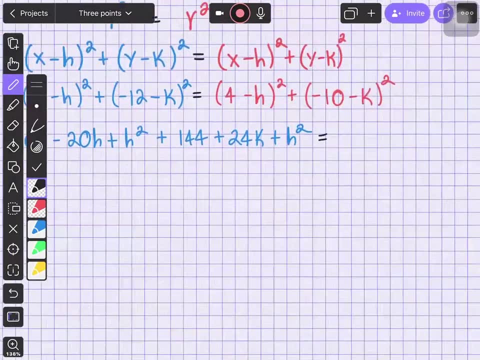 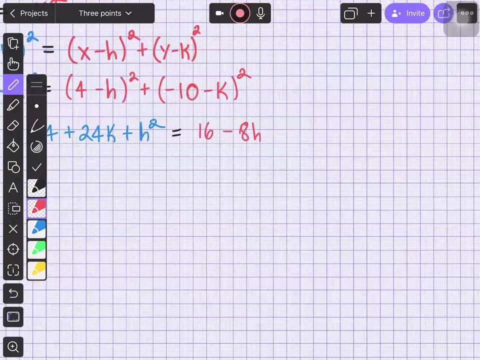 and this one over here is the second one, so i have my blue side ready and these will be equal to- sorry, let's begin: four squared four times two, and then h squared. all right, this is just the first one, sorry. now negative 10 squared 10 times 2. 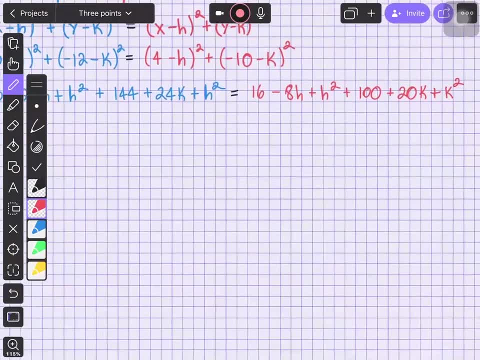 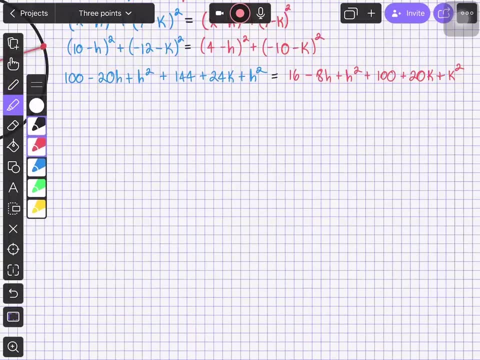 and k squared. there we go. so if you see, in this equation, this log equation, we have the square variables h. this one should be okay there. all right, sorry, this is k, both h and k on both sides of the equation, so they will cancel each other out. so now, 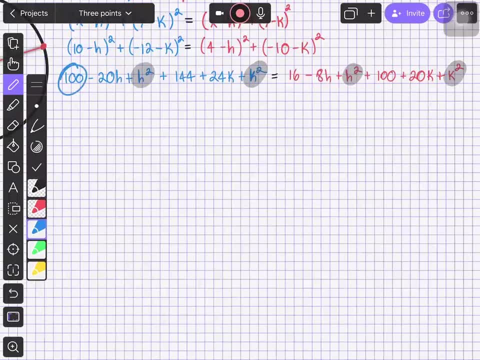 we can add 100 and 144 and have a shorter equation. so 100 minus 20 h. now let's do the addition right now. now let's save some steps. 244 minus 20 h plus 24 k. okay, and we can do the same over here: 16 and 100, it's 116 minus 8 h plus 20 k. 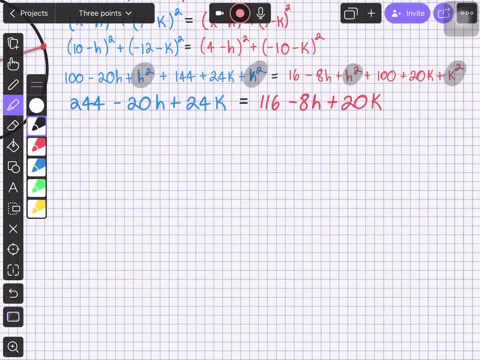 now, from here we're going to leave the variables right, these ones here on the left side of the equation and the numbers on the right side. so we have negative 20 h plus 8 is negative 12 h. now 24 k minus 20 will be 4k and 116. 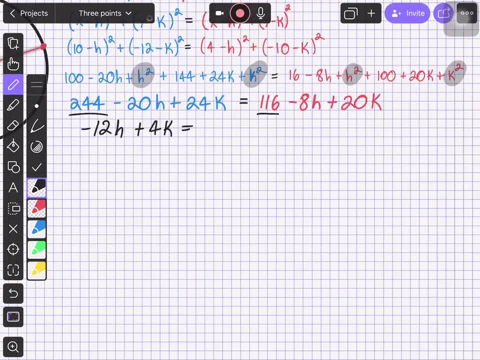 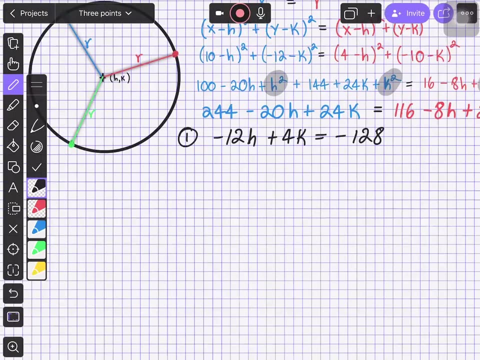 minus 200, 44 will be negative 128. this is our first equation. so if you see, we have a linear equation with our variables h and k, the center, as the only two variables, right? that means that we have to do the same process again to come up with the same result. so we have to do the same process again to come up. 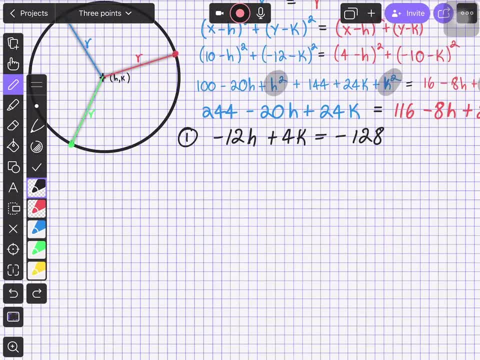 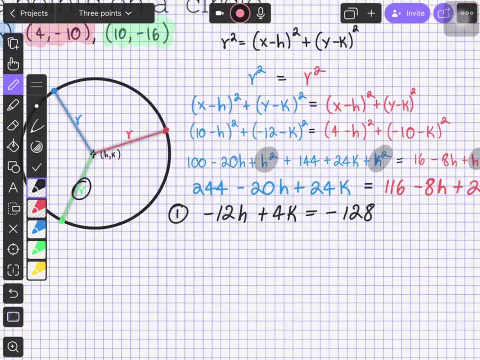 with a second equation that we can use and solve as a system of equations. so that means that instead of the blue one now, we will have to use the green one. all right, so let's use the, the green and the red. it doesn't matter which ones you select, it's just. 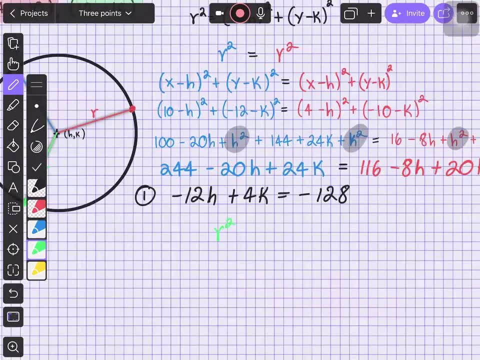 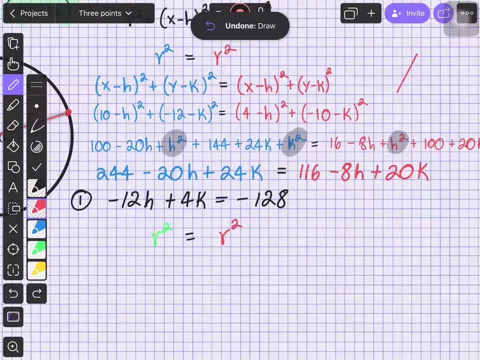 the ones i am selecting right now. so same idea: the green square radius will be the same grew as the red square radius. now here's- uh, there's- a good news. you already have the red side developed, so you just have to develop the green side. all right, you just have to copy that. 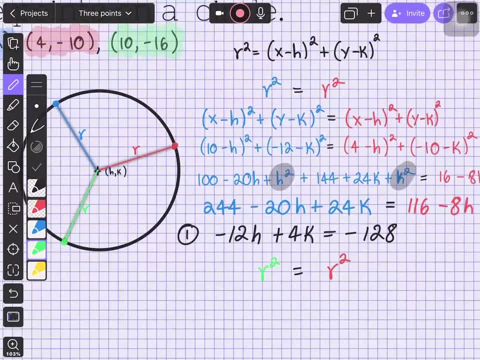 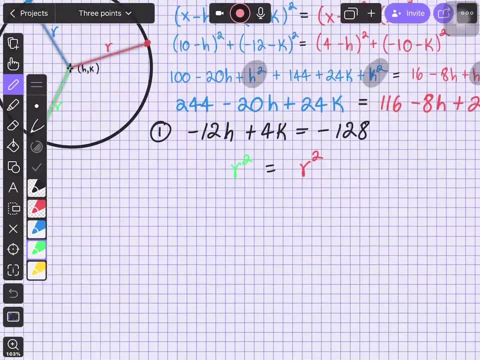 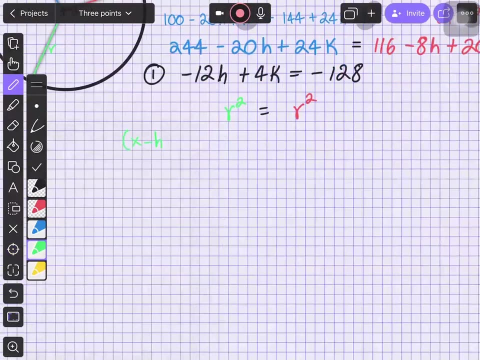 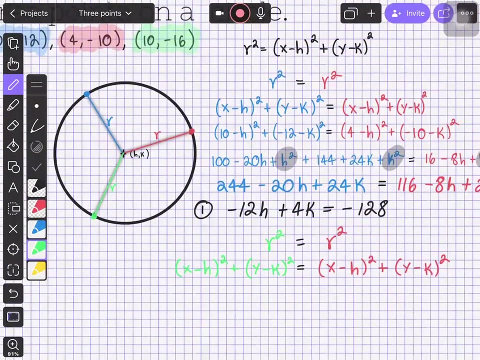 the red part of the equation. so let's see 10 negative 16.. all right, sorry. so our equations x minus h squared plus y minus k squared equals x minus h squared plus y minus k squared. all right, now, now the substitution. i'm sorry. now yes, 10 and negative 16.. 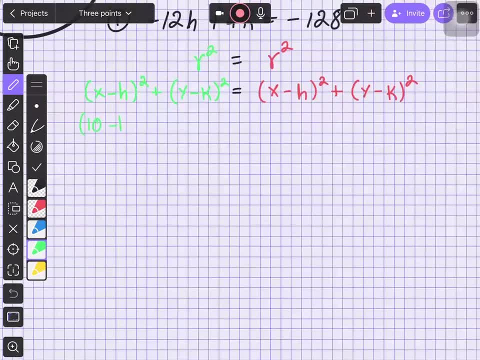 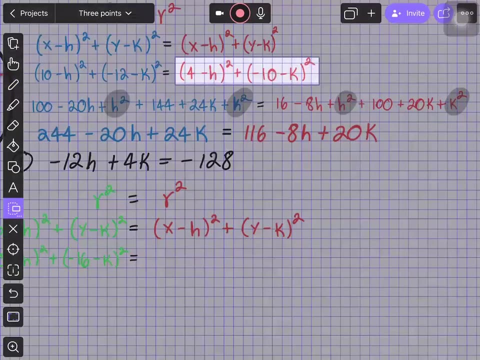 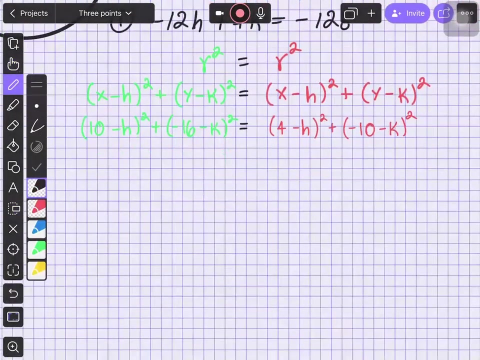 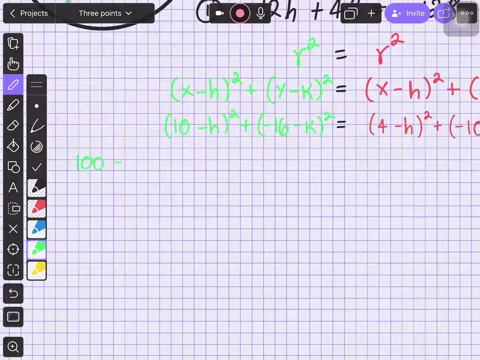 all right, 10 and negative 16.. now this one, we already have, it's over here, all right, so we just copy it all. right now let's develop the green side. let's expand the binoms. we have 100 times 2, and then I square, 16 is 256, times 2, 32k and k squared, and this expansion. 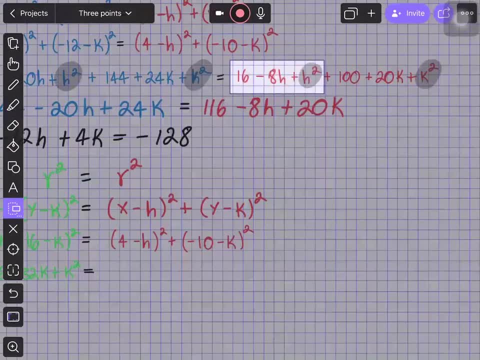 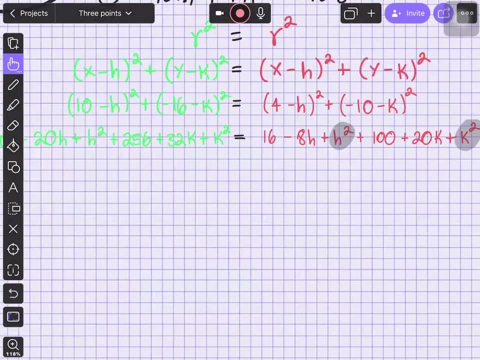 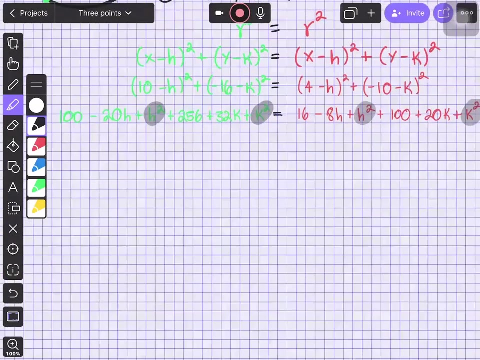 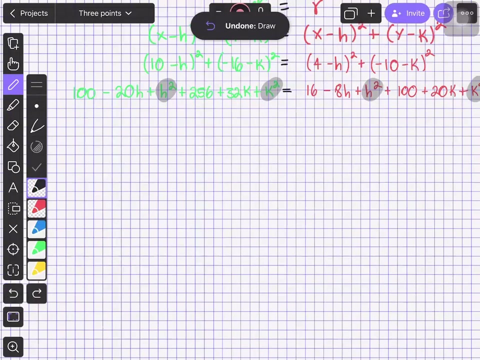 we already have here. it is now. if you see, in this expansion the k and the h are cancelled because again we have them on both sides of the equation. so now we can add the numbers. all right, 100 and 256, we have 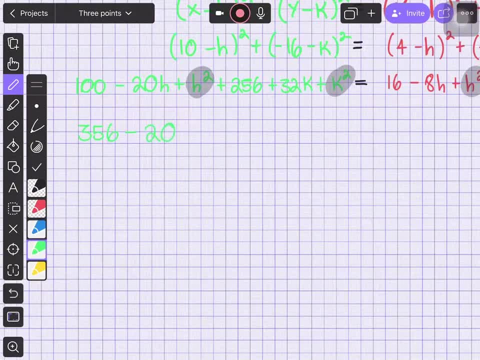 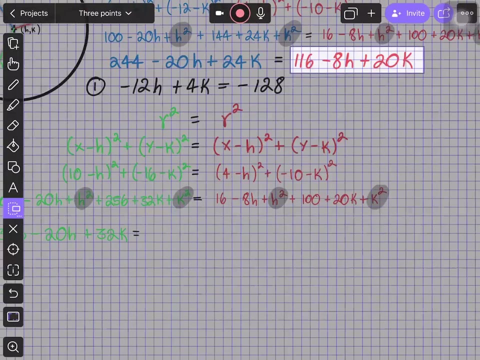 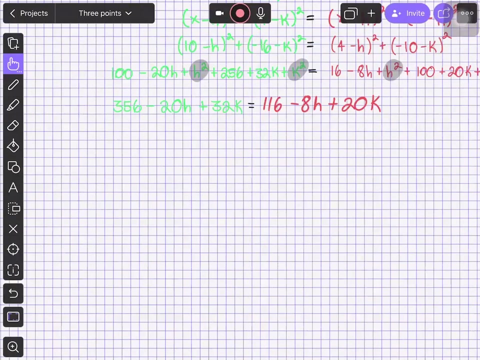 300, 356, minus 20h, plus 32k, and this equals, and we already have it all right. there we go and now, yes, same as this as before: the variables okay, on the left. 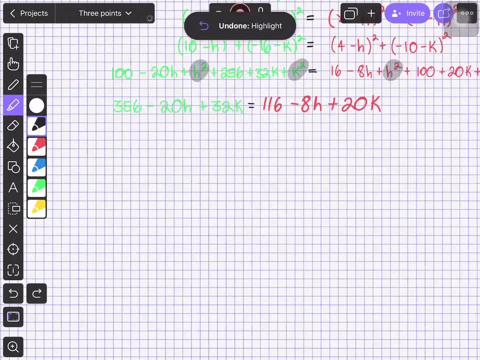 side of the equation and the numbers on the right side. so negative 20h, all right, plus 8,- sorry- is negative 12h, all right. 32 minus 20 is plus 12,, okay, and 116 minus 350,. 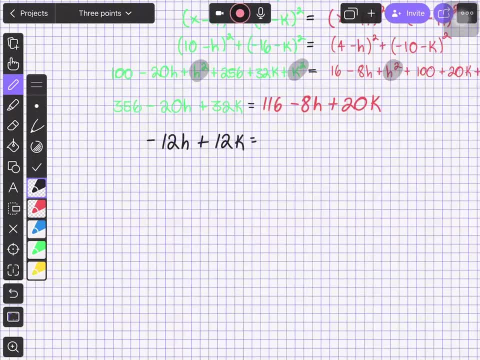 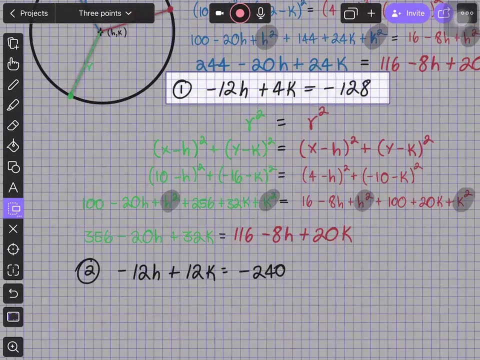 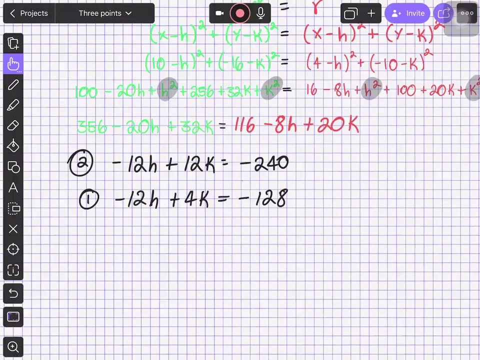 156,, 0,, 4,, 240,, negative 240,, and this is our second equation. all right, so now we bring our first equation, and now you see, we can solve it. all right, let's multiply the first equation. 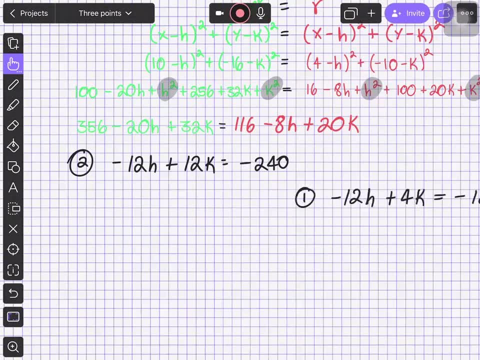 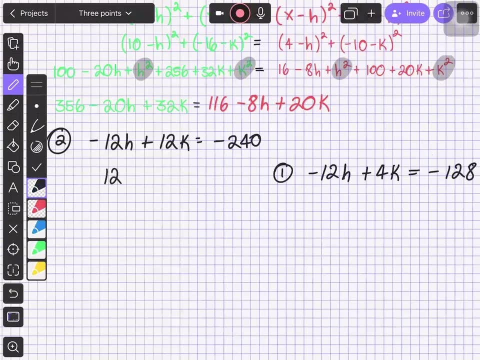 times negative 1,. let's put it over here, so we will have: 12h minus 4k equals 128,. all right, we can do the addition now. this will get cancelled and 12 minus 4 is 8k. 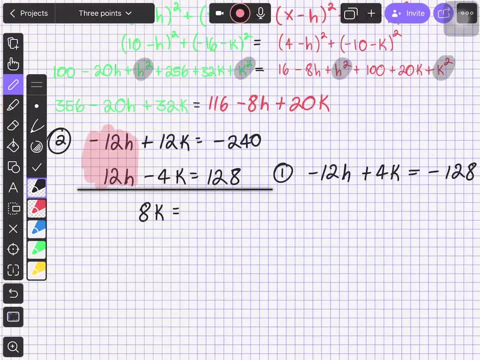 and 12 minus 4 is 8k, and 12 minus 4 is 8k. all right, give me one second: 240 minus 128,. no wait, getting lazy with the calculator. 112,, all right, negative 112, so k will be 112,. 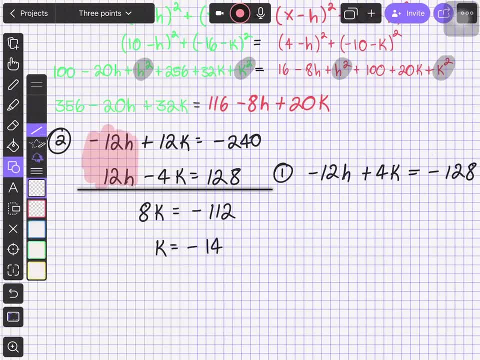 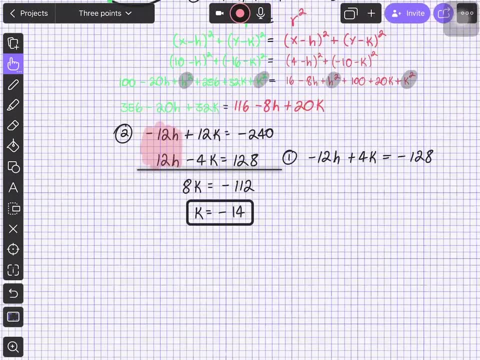 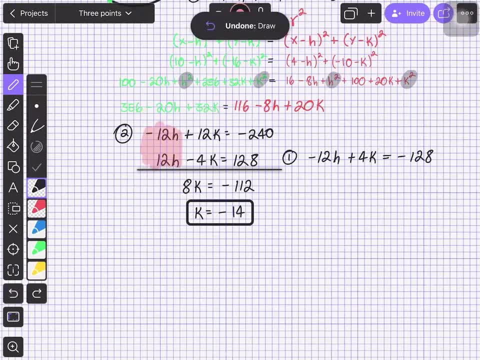 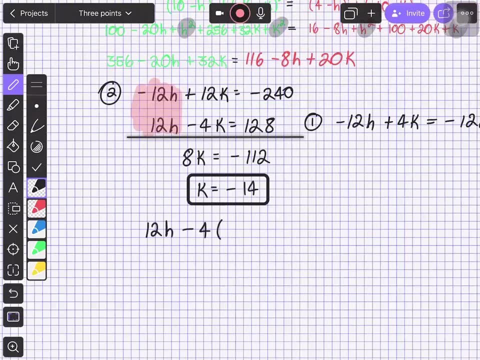 substituting here. all right, to make it easier. so we will have: 12h minus 4 times negative, 14 equals 128,. 12h will be 128 positive, negative, 56, 100,. give me just one second: 128 minus 56 is 72,. 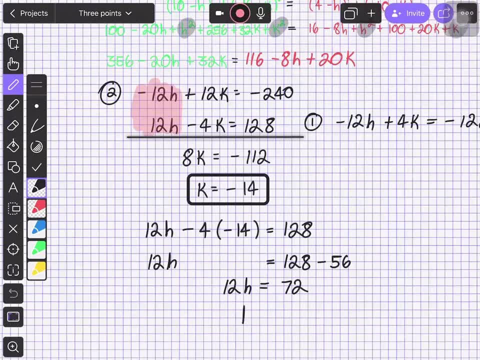 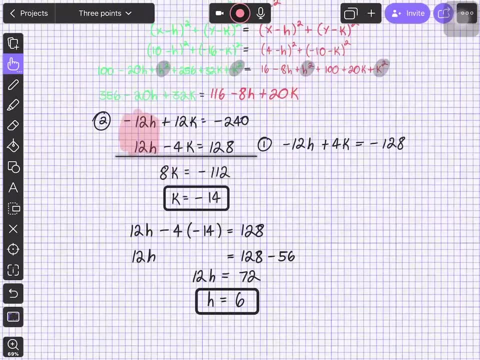 and 72 divided by 12 is 6, so now we have the second one. so now we have the second one. so now we have the second one right. and in the third example let's use thezen俺 cancel out. 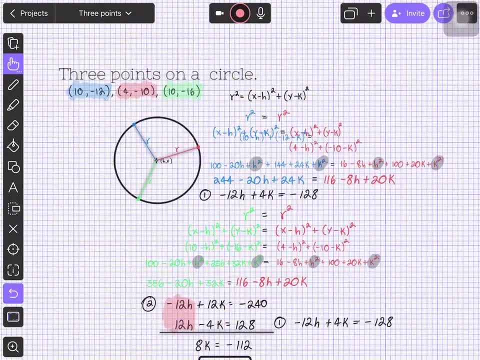 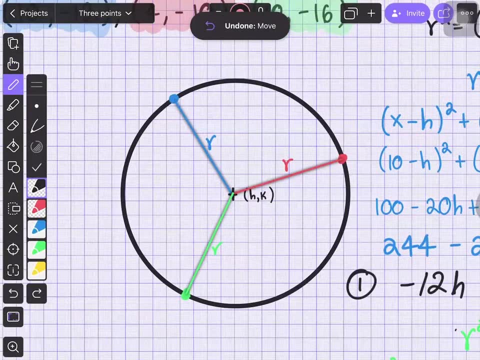 and in the third example, all right, nine, five and seven, and we subtract and we subtract, which is seven. now we should be able to. therefore we have the center, all right now, if we go back here. 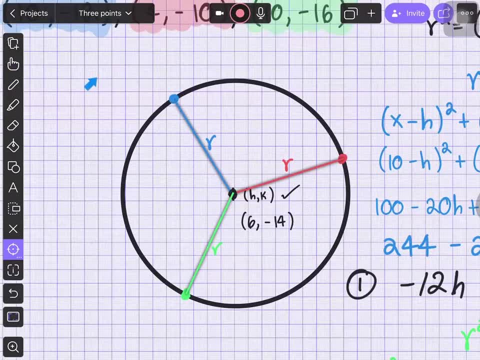 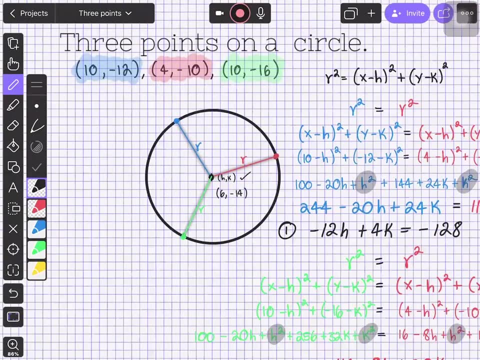 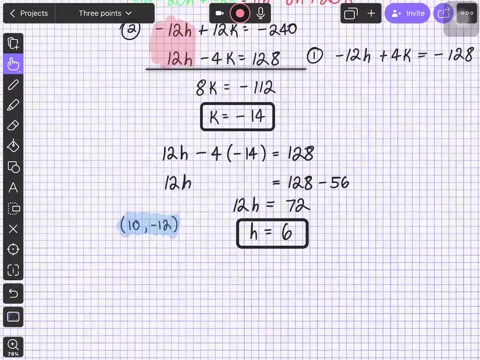 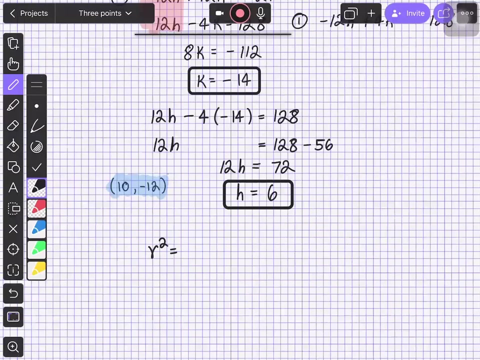 sorry to calculate the radius squared and we will be done so which one looks. okay, that's exactly the same. let's take this one, get over here points. so the radius squared will be X and Y and we have H and K, so X minus H squared this. 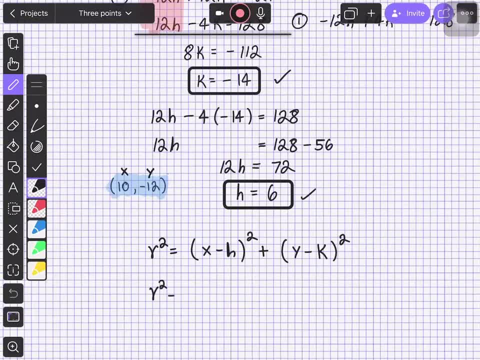 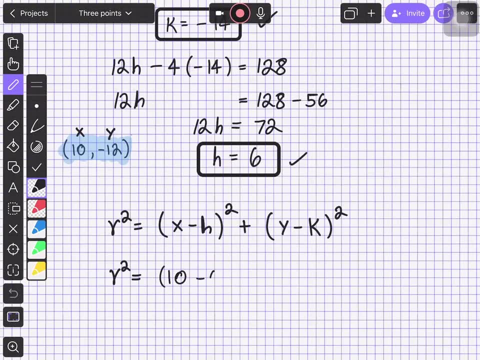 Y minus K squared, so the radius squared will be 10 minus X squared, plus negative 12 minus negative 14 square. this is 16, and this is 2 and 4. 16 and 4, this is 20. there we go and we're done, and now we can write.